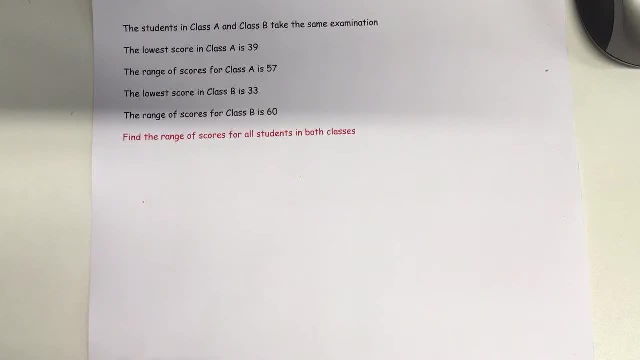 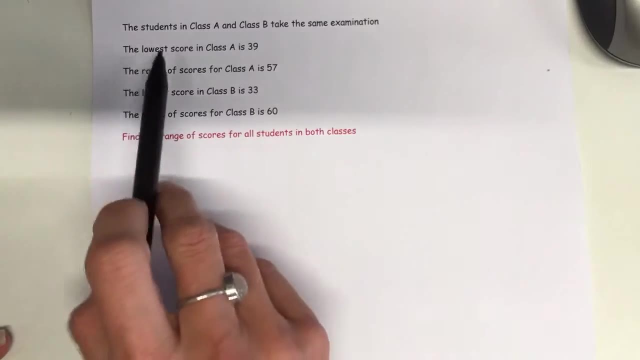 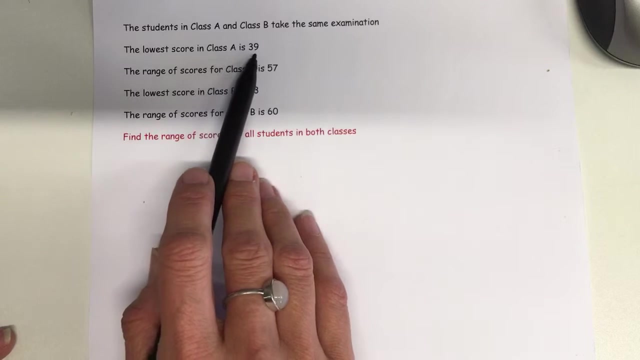 This video is going to look at problem-solving involving the range. So we're given quite a bit of information in this question. We're given that the students in class A and class B take the same examination and we're given the lowest score in class A is 39 and the range of the scores in class A is 57. So 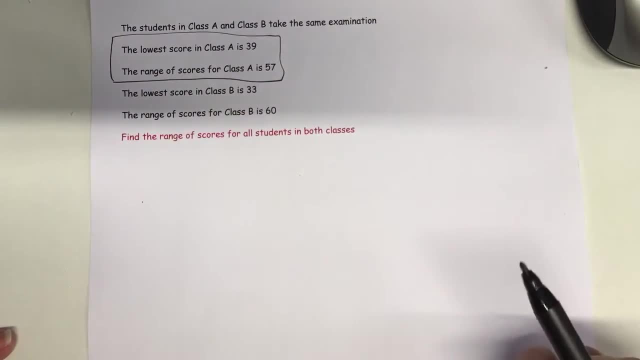 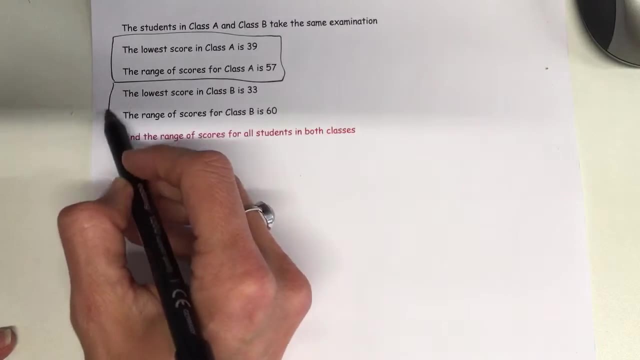 we can think about those two pieces of information together and then we're given the lowest score in class B is 33 and the range of the scores in class B is 68. So we would block those two bits of information together as well And we 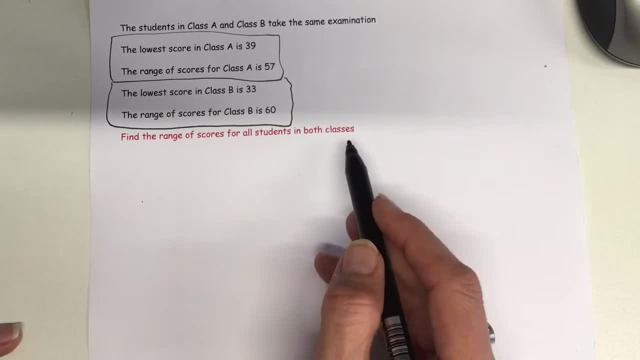 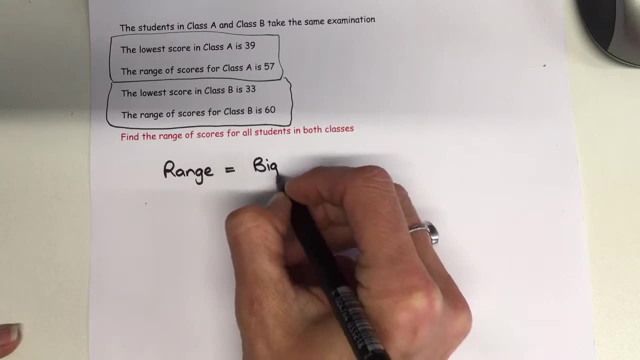 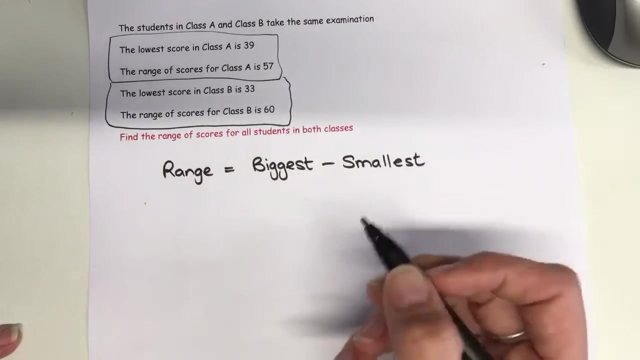 need to find the range of the scores for all students in both classes. Now, when we talk about the range, we are thinking about the biggest number subtract the smallest number, And for class A we are given that the lowest score is 39, so we're given this number here, 39. We don't. 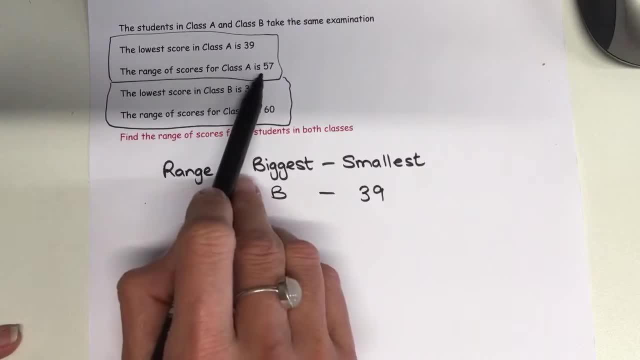 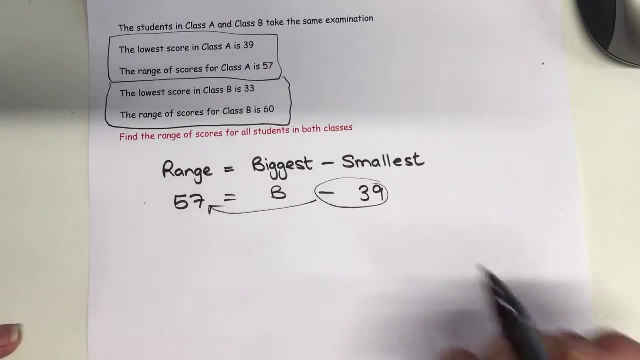 know what the biggest score is, so I'm going to call that B, And we're given that the range is 57. So to find B I must add that onto 57. So B is 57 plus 33, which is 96.. 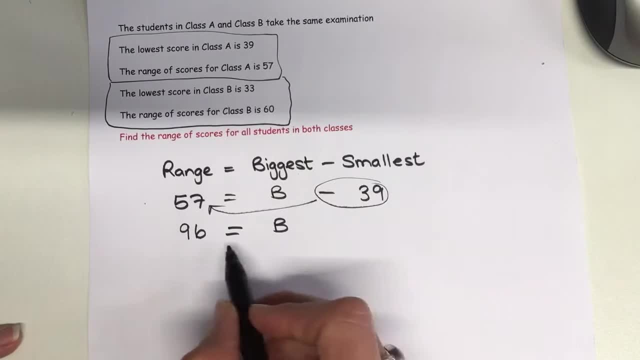 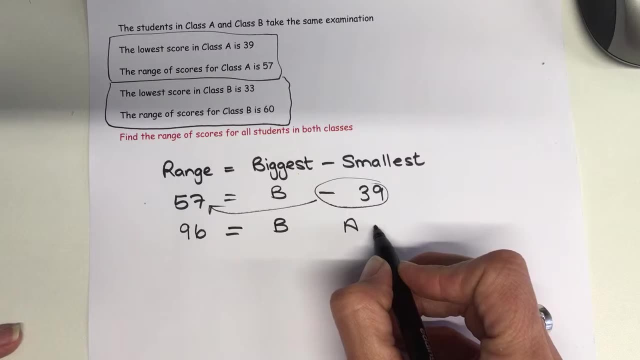 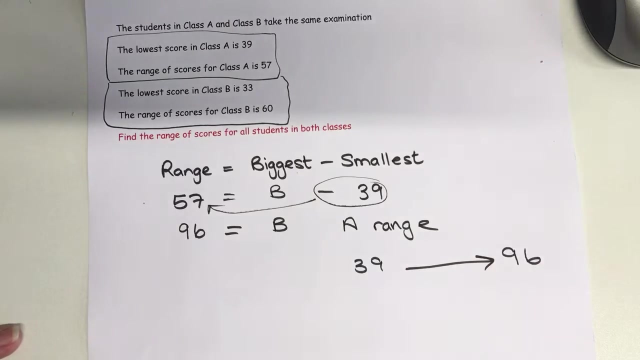 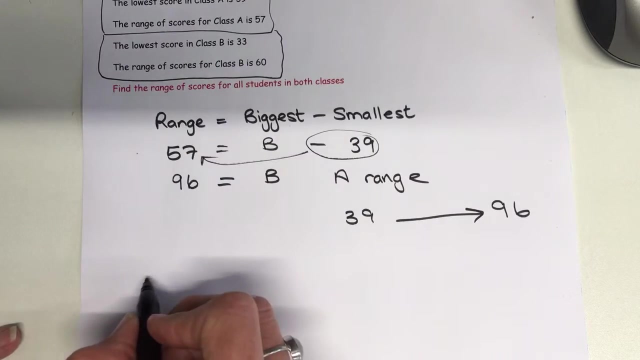 So the biggest number in A is 96. So in A the numbers range from the smallest number at 39, right up to the biggest number, which is 96. Now if we move on and we look and we apply the same thing to the score for B, then again range equals. I'm going to put B, I'm going to use. 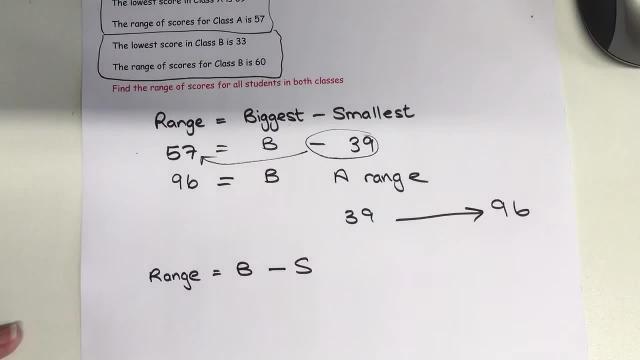 B instead for minus S. big takes small this time, And we are given that the range for B is 60. And we're given the lowest number is 33.. So we don't know what the biggest number is, but we know the smallest number is 33.. And again, we are going to read that as well.